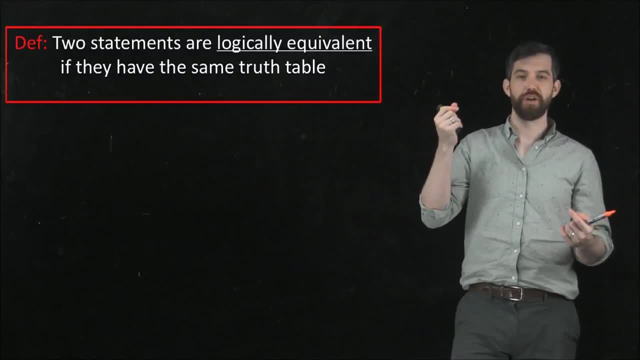 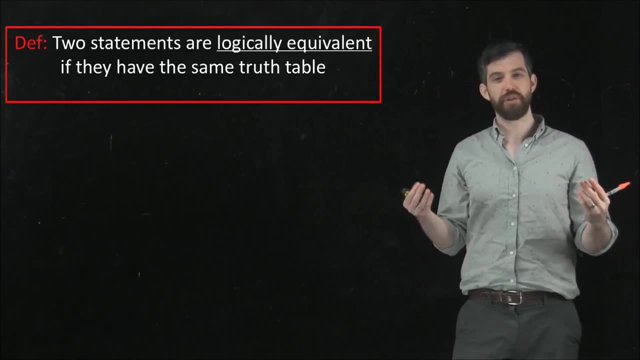 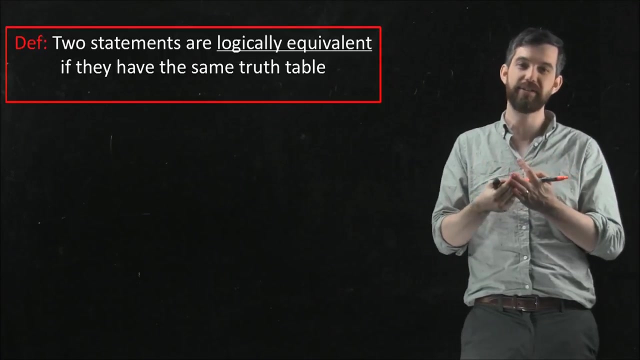 The next concept we want to introduce is that of logical equivalence between two different statements. Now the idea here is that you could have two statements and both of them could be really long, messy, compound statements have got lots of ors and ands and nots and all sorts of different inputs, and it's not clear. 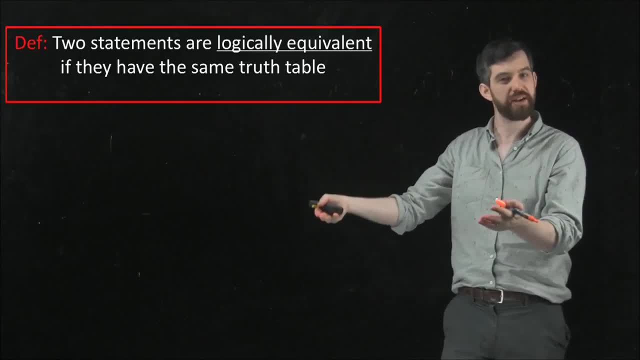 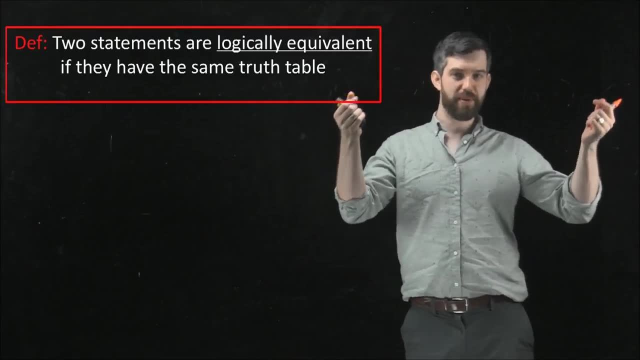 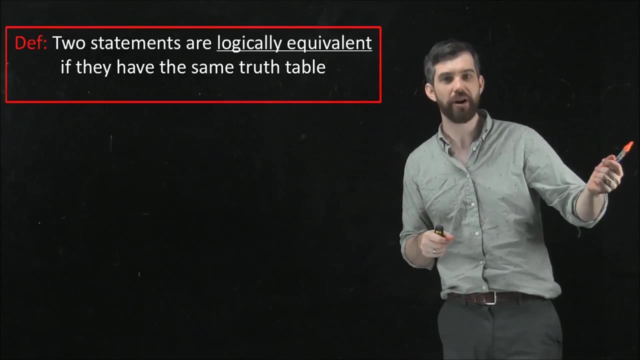 whether those two statements are the same thing but just presented differently, or whether they truly are different things, and the way we're going to claim that two statements that maybe superficially do not look to be the same are in fact logically equivalent. if you have one, you get the other. we're gonna. 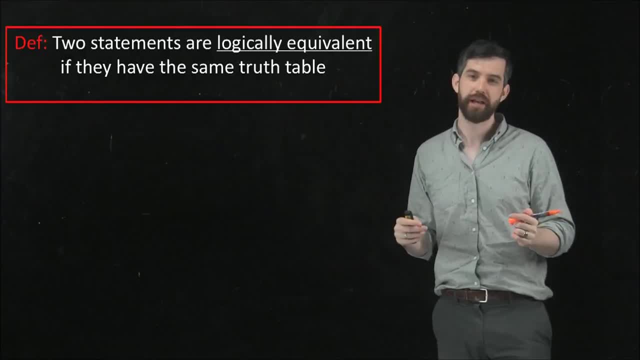 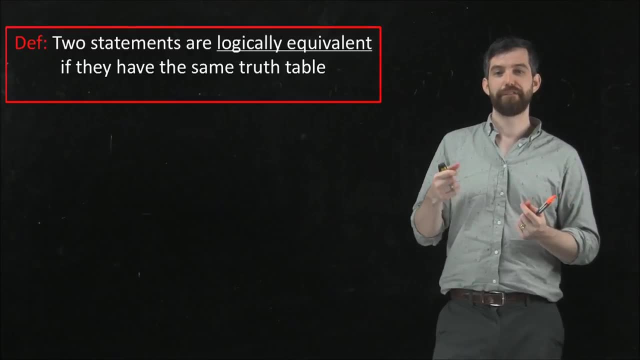 say they're logically equivalent if their truth tables are identical, which is to say we're saying something is logically independent or logically equivalent, rather, if it's the case that for every pairing of their inputs, all true false pairings of their P's and their Q's. 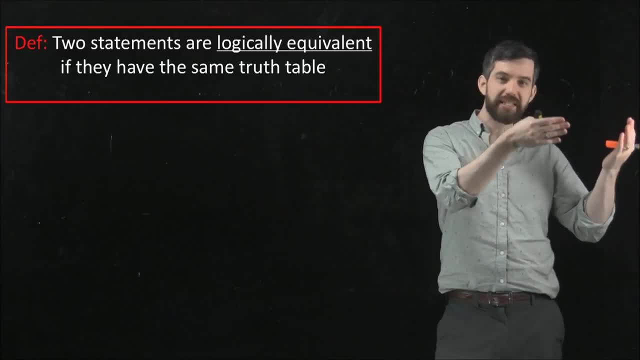 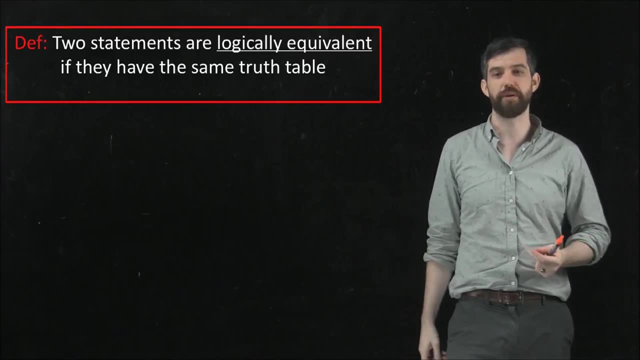 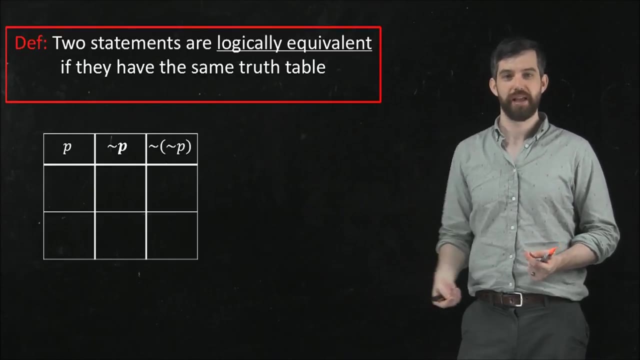 that their output is going to have the exact same truth and falseness for every different possible input. so that is our idea: is having the same truth table. so here's a simple example. I want you to look at the statement, not not P, and, and we know that this idea of a double negative, is that a double negative in? 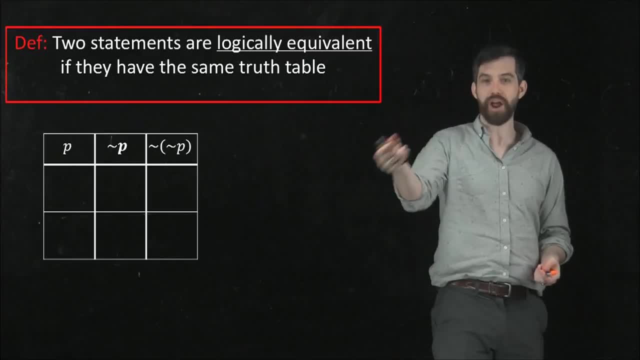 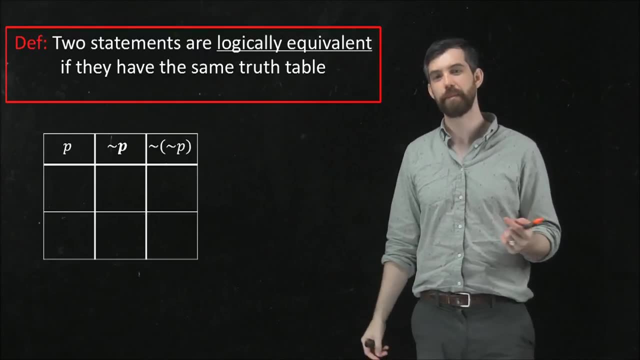 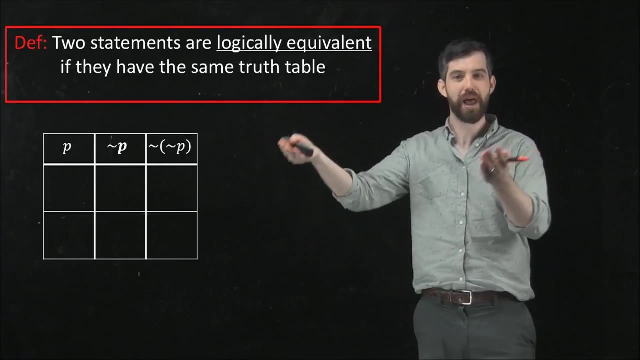 English sort of cancels, right, if I say that I am not not hungry, and that's me saying that I'm hungry, but if I put a double negative in, you can sort of imagine it canceling. now let's just try to verify that, that this actually makes logical sense, according to what I've told you. 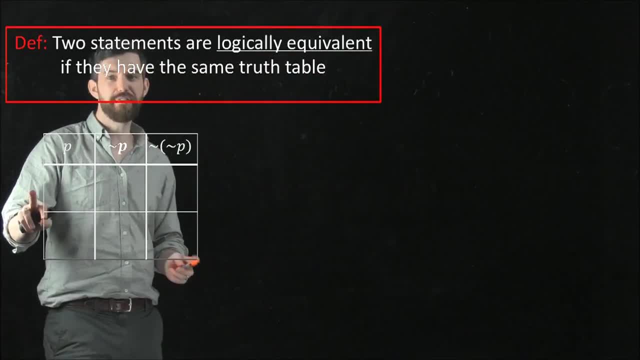 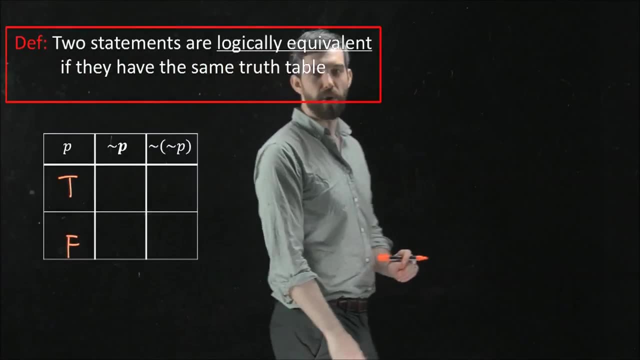 which is the truth tables. so first of all, we're going to go in and we're going to try to fill in what's happening here. for P, my two different inputs are true and false, so I always do that first I put all of the possible input values. 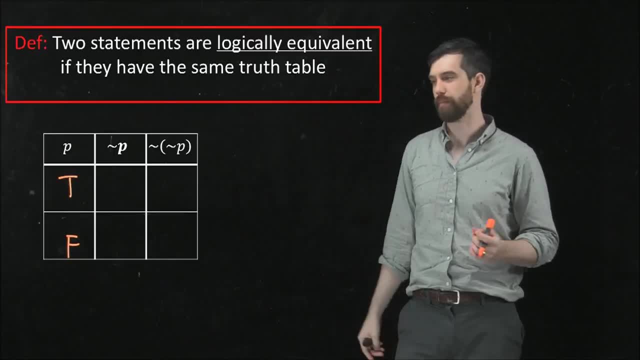 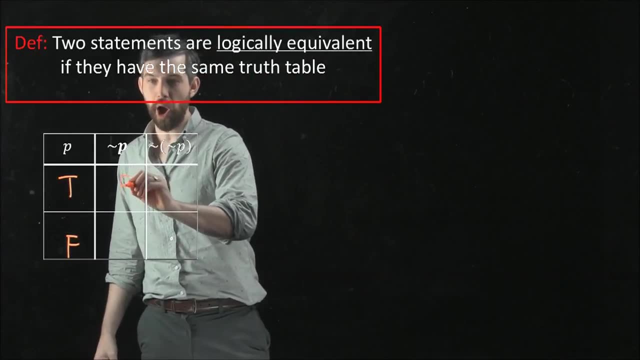 that I could have my truth or falseness of that input P. so then, if I look at not P, which is just sort of an intermediate step here, if P is true, then not P is going to be false, and if P is false, then not P is going to be true. so